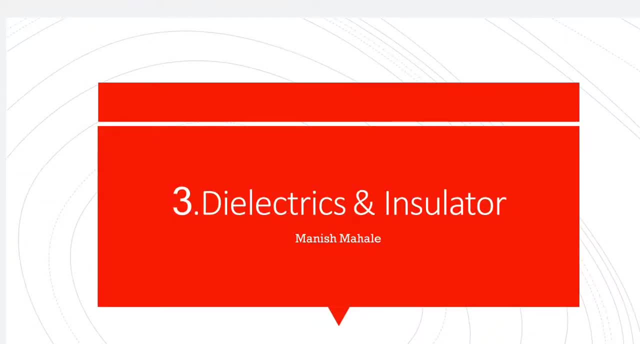 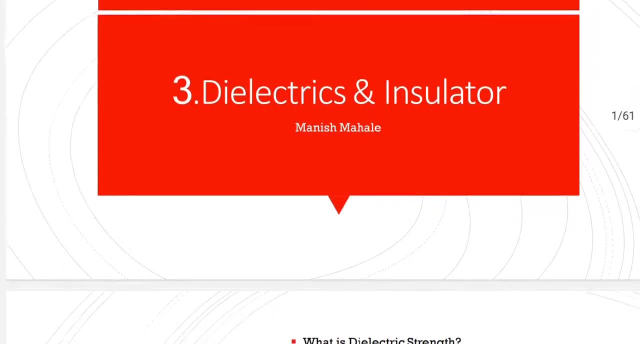 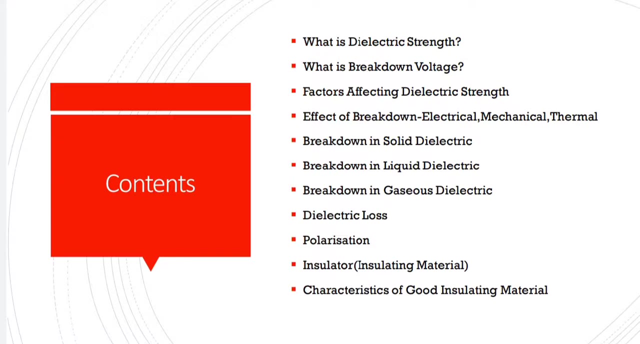 Hello, friends, welcome all. so in this video we will discuss the third chapter, dielectric and insulator. in this third chapter we will discuss about what is dielectric strength, what is breakdown, voltage, its, what are the factors affecting dielectric strength? then effects of breakdown, that is, electrical, mechanical and thermal effect. then breakdown in solid. 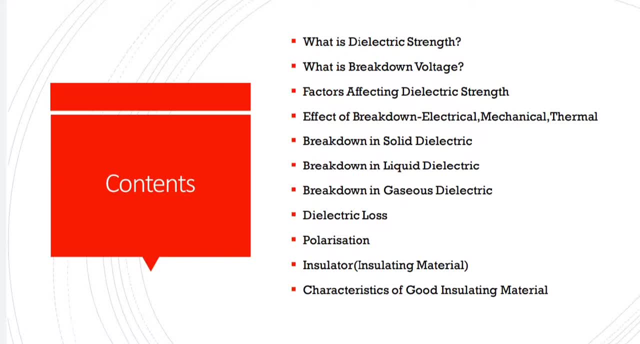 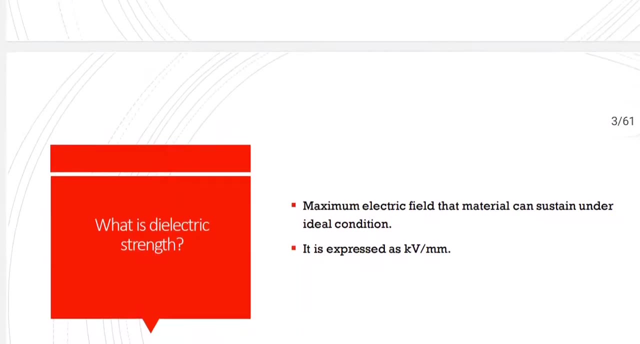 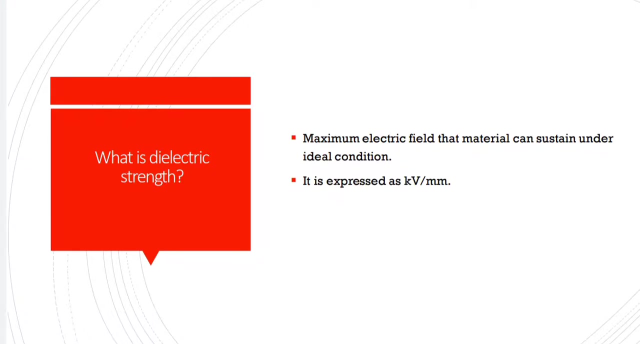 liquid and gases, dielectric, dielectric loss and polarization. and, last but not least, insulator- insulating material and its properties and characteristics of good insulating material. okay, so let us discuss about what is dielectric strength, but before we should define dielectric strength, we should discuss about what are dielectric and what are insulating materials. 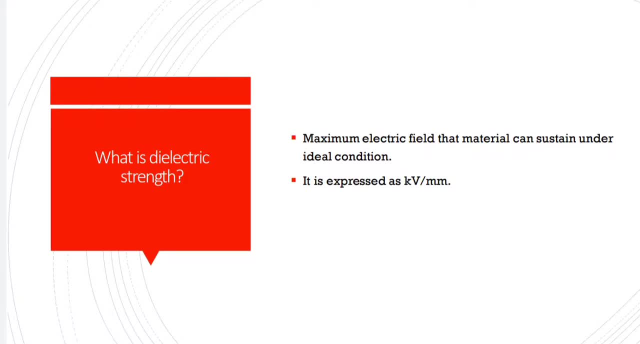 so dielectrics or the insulator are the distinct form of conductors which does not have any free electron. okay, so the material which does not contain the moving electrons are called as dielectric or insulating material. hence, when a source of emf is connected across the dielectric, no current flows. 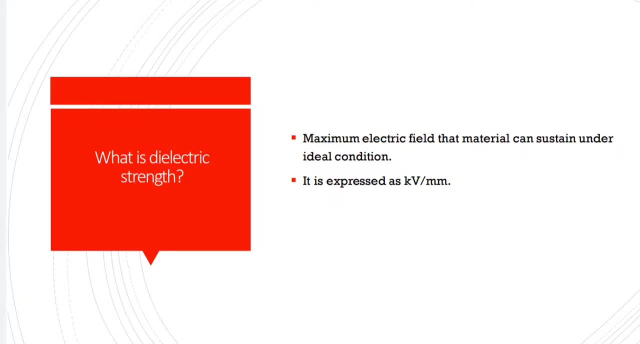 means when, if we apply the voltage between the two points of the dielectric and the insulator, then the dielectric will not have any free electron of the dielectric material, then there is no current flows, that is, no free electrons is present in that material. however, since no dielectric is perfect, it contains a small 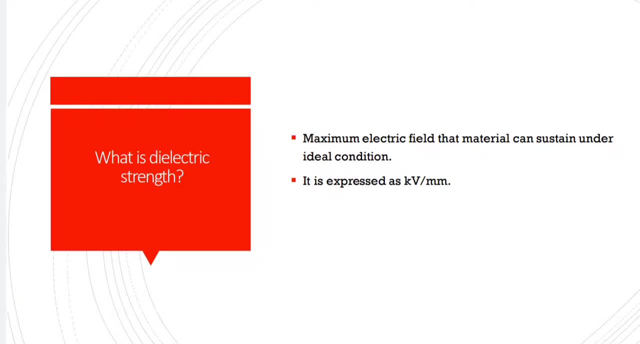 number of free electrons and a very small current flows through it when electric field is applied between two points of the dielectric material. so this is called as capacitor effect or capacitance effect. capacitor, therefore capacitor, have a small leakage conductance in in it. okay. so dielectric, best dielectric example is capacitor. so dielectric materials are essentially 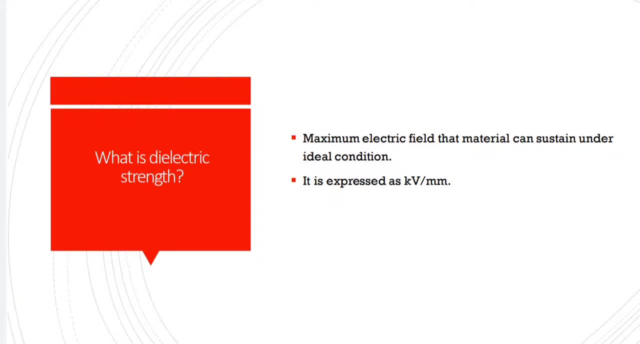 insulating materials. however, while the function of an insulating material is to obstruct the current flow and the function of dielectric material is to store the energy, there is a small difference between dielectric and insulating material. that insulating material does not allow flow- the current- but dielectric material can store the charge or store the energy. 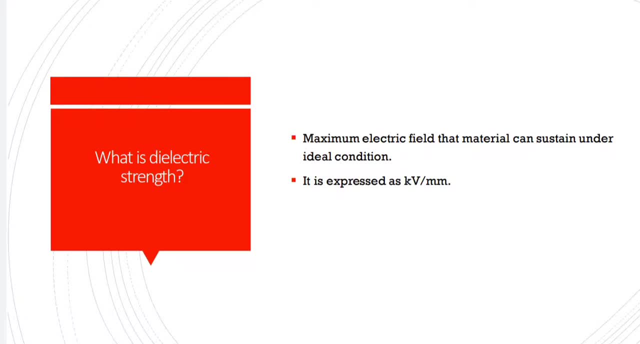 in it. so there are three types of dielectric materials, that is, solid dielectric material, liquid dielectric material and gaseous dielectric material. okay, so I hope that you would understand what is dielectric and what is insulator. there is a one major difference is that all dielectric materials are insulator. 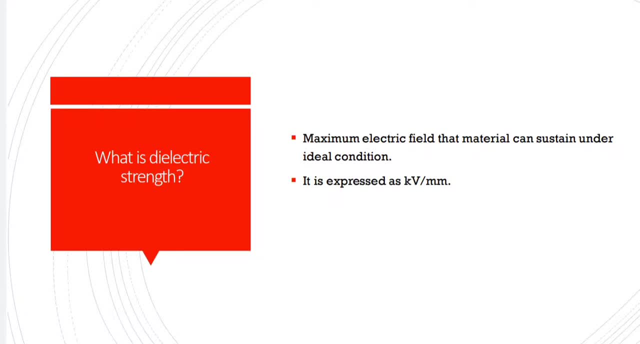 but all insulating material are not dielectric material. so remember that and that all insulating materials are dielectric material. sorry, all dielectric materials are insulating materials, but all insulating materials are not dielectric material. okay, so this is. I hope that you have understood the difference between. 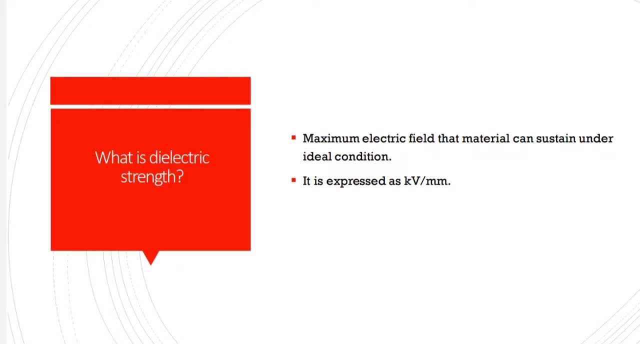 dielectric and insulating material. okay, so let us now discuss what is dielectric strength? so dielectric strength is nothing but maximum electric field that material can sustain under ideal condition. or you may be defined the dielectric strength is. it is a ratio of breakdown voltage to the thickness of the dielectric. okay. the intensity. 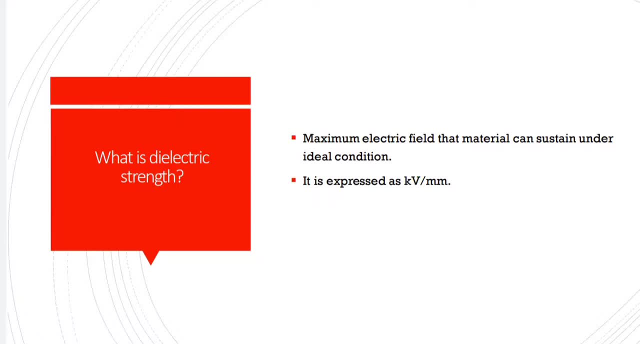 of the electric field at which breakdown occurs is called dielectric strength. it is generally expressed in kilo volt per mm. kv per mm- okay, where kv is kilo volt and mm is area of the thickness of the dielectric material- okay, and kv is breakdown voltage. okay, so now again question. 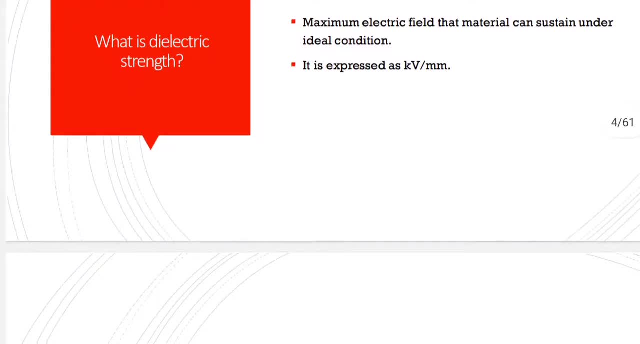 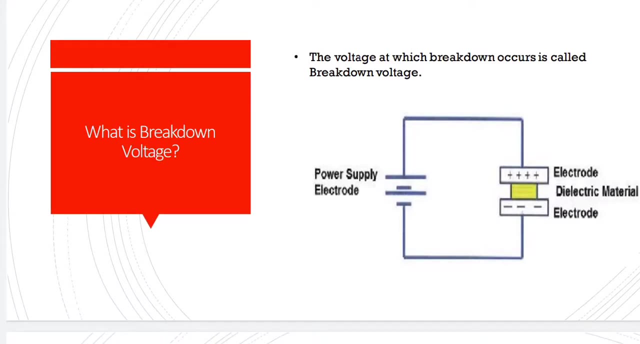 arises. what is breakdown voltage? what is breakdown voltage? so let us discuss what is breakdown voltage if the voltage across the place- let's see the figure uh which is shown on the slide. okay, so if the voltage across the plate is increased slowly, a stage is reached at which the dielectric breakdown and short circuit, short circuiting. 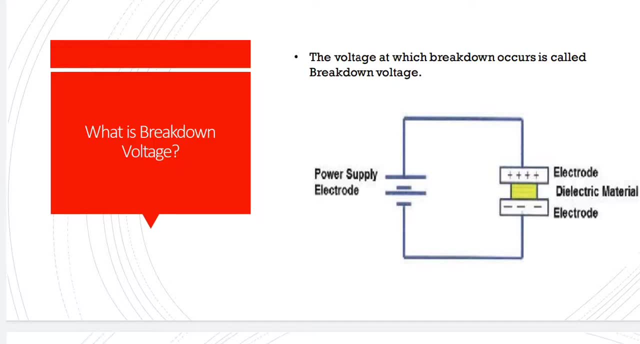 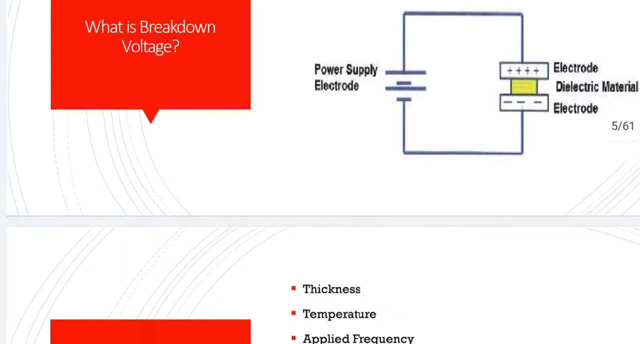 of the plates causes the voltage at which breakdown occurs is called breakdown voltage, where, when there is a short circuiting occur between the both plates, the voltage, the point at which the voltage at which the breakdown occurs, is called breakdown voltage. so there are some factors, uh, on which dielectric strength depends. so the factors are: thickness,